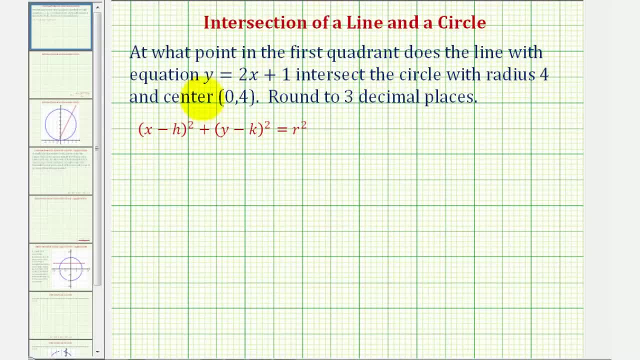 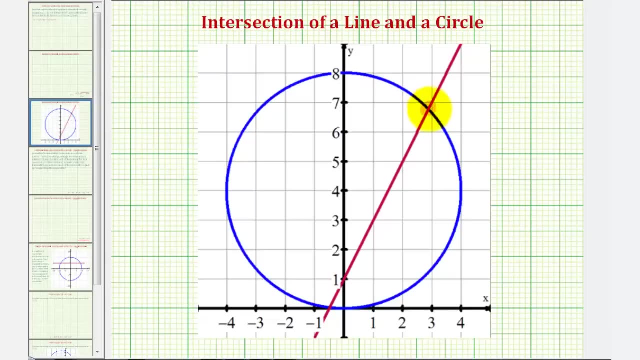 At what point in the first quadrant does a line with equation y equals two x plus one intersect the circle with radius four and center zero, comma four, And we're asked to round to three decimal places. So graphically we're looking for this point of intersection here in the first quadrant. We take a look at the line. 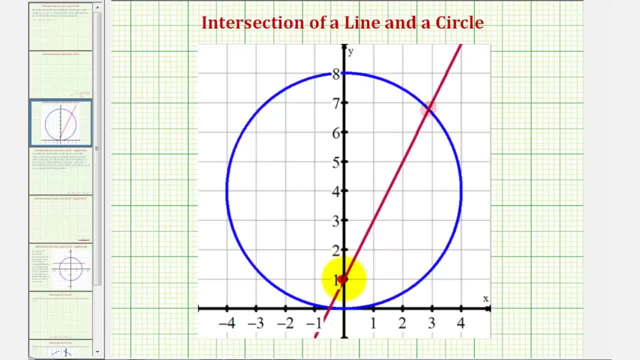 first, Notice how it does have a y-intercept of positive one and from here, if we go up two units and right one unit, we're still on the same line, verifying the slope is positive two. Then, looking at the circle, notice how it has a center of zero four and the radius is four units. So we're going to begin by 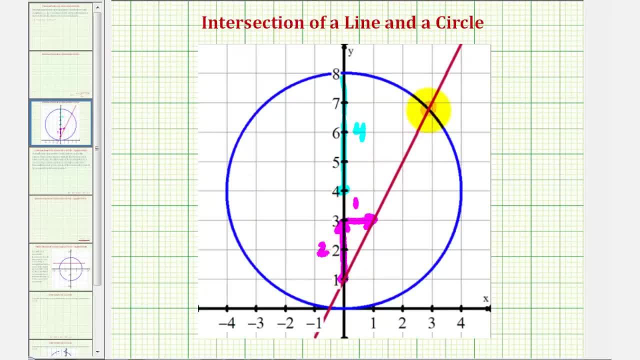 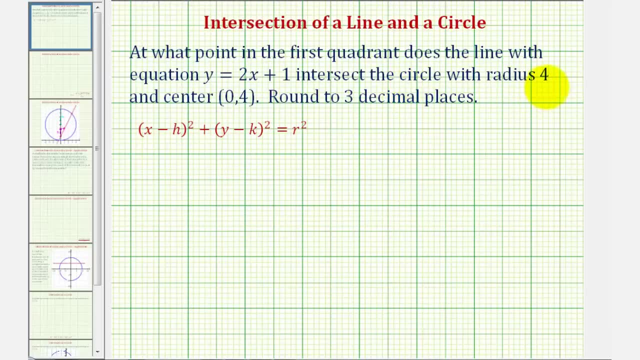 determining the equation of the circle and then solve this as a system of equations. So using this equation of a circle, because the radius is four and the center is zero, comma four, h is zero and k is four, Which means the equation of the circle would be the quantity x minus zero. 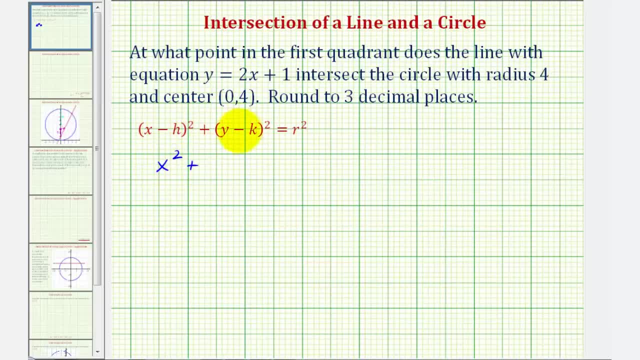 squared, or just x squared plus. again, k is four. so we have the quantity y minus four squared equals r squared, which would be four squared or sixteen. Now we know the linear equation is: y equals two, x plus one. So again, we're going to solve this now as a system of equations. We're going to 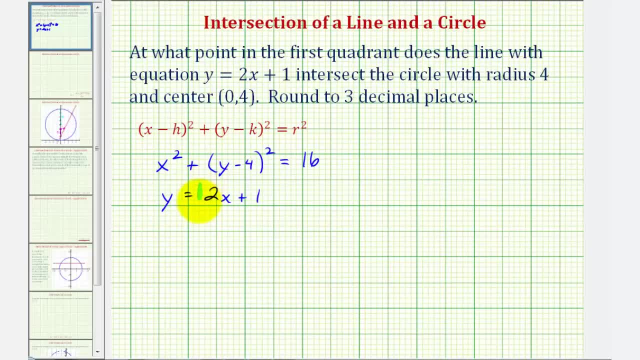 use substitution Notice: here y equals two x plus one, so we'll make the substitution for y in the first equation. We'll substitute to two x plus one here for y. So this would give us the equation x squared plus the quantity two x plus one minus four. 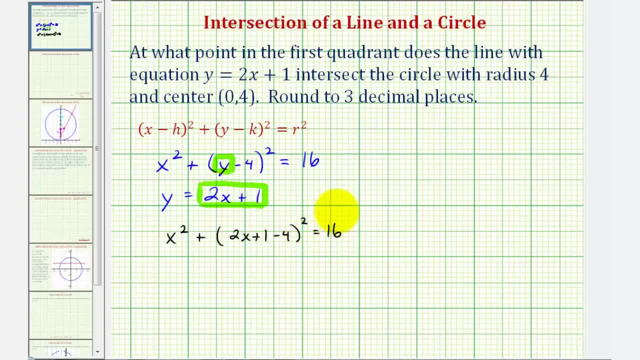 squared equals sixteen. Let't go and simplify this. We'd have x squared plus the quantity two x. this would be plus one. minus four is minus three. squared equals 16.. Notice, now we have an equation with one variable, So now we'll expand this. combine like terms: 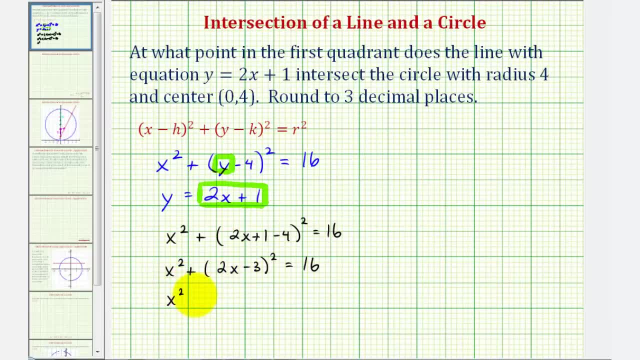 and solve the equation. So we'll have x squared plus the quantity two x minus three times the quantity two x minus three equals 16.. Here we'll have four products: one, two, three and four. So we'll have x squared and then plus four: x squared. 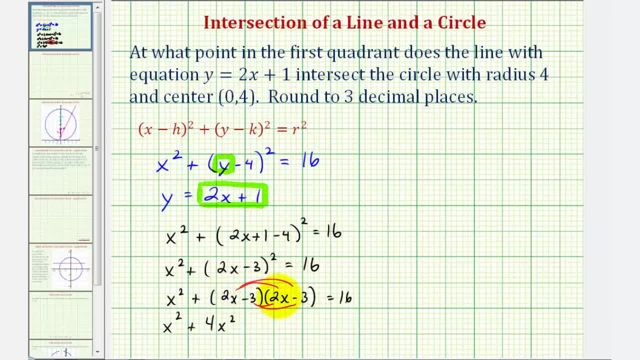 The next product would be minus six x, but then we have another minus six x, that's minus 12 x, and then plus nine X squared, plus four x squared, would be five x squared. Then we have minus 12 x. plus nine equals 16.. 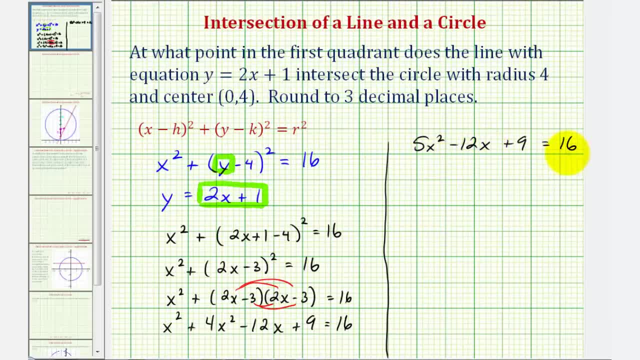 We have a quadratic equation, so we're going to set it equal to zero and see if it factors. So we'll subtract 16 on both sides. That would give us five x squared minus 12 x If we subtract 16 on both sides. 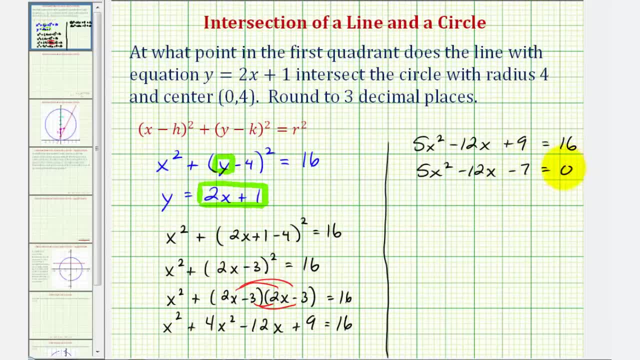 that's going to give us minus seven equals zero. Unfortunately this is not factorable, so now we'll have to solve this using the quadratic formula. And keep in mind we're looking for the point in the first quadrant, so we're only concerned. 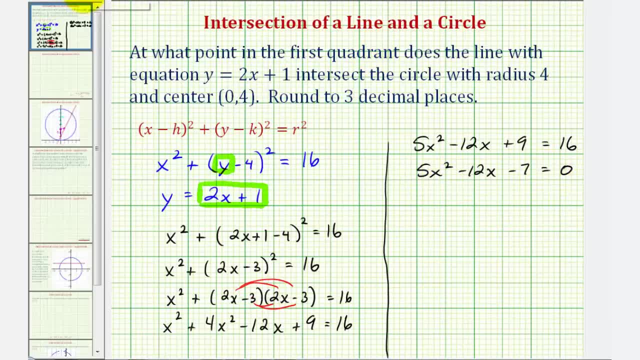 about the positive solution to this equation. Remember, when using the quadratic formula, we'll have a equals five, b equals negative 12, and c equals negative seven. Keep in mind we are asked to round the coordinates of the point of intersection to three decimal places. 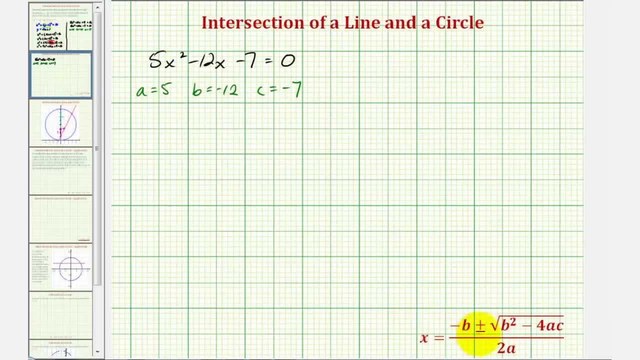 Let's go ahead and solve this on the next slide. Here's the quadratic formula. if we need to review, We would have x squared plus six x squared minus six x squared, We would have x squared minus six x squared minus six x squared. 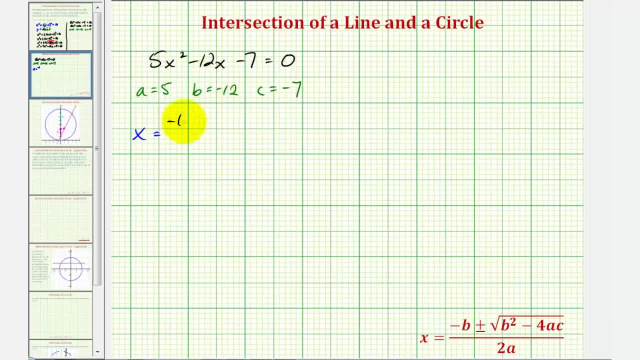 We would have: x equals negative, negative 12 plus or minus the square root of b squared, That's negative 12 squared minus four times a, which is five times c, which is negative seven. We'll divide all of this by two times a, or two times five. 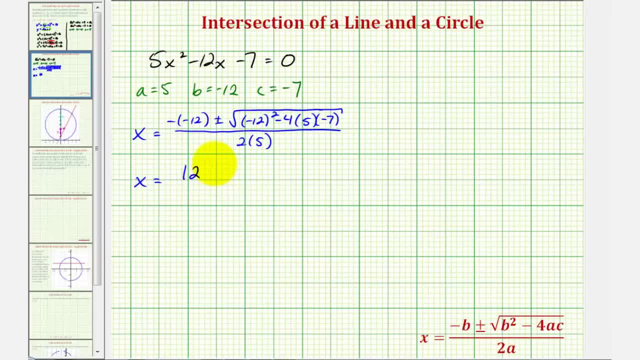 So we have: x equals positive 12 plus or minus. the square root of this would be 144 plus 144.. That's 284 divided by 10.. Now we don't need to simplify this, because we're looking for a decimal value rounded to three decimal places. 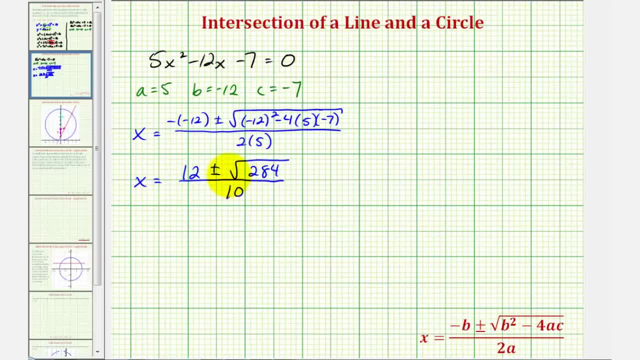 But we are looking for the positive value of x in the first quadrant, which means we're looking for the decimal approximation, for x equals 12 plus the square root of 284 divided by 10.. But just in case you were curious, 284 is equal to four times 71.. 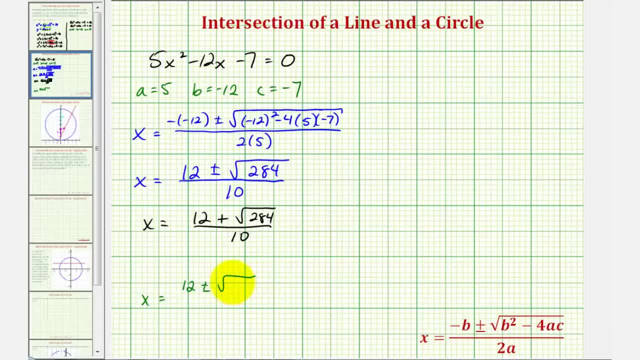 So that would be 12 plus or minus the square root of four times 71 divided by 10, or 12 plus or minus two square root of 71 divided by 10.. And then, to simplify this, we could break it up into two separate fractions. 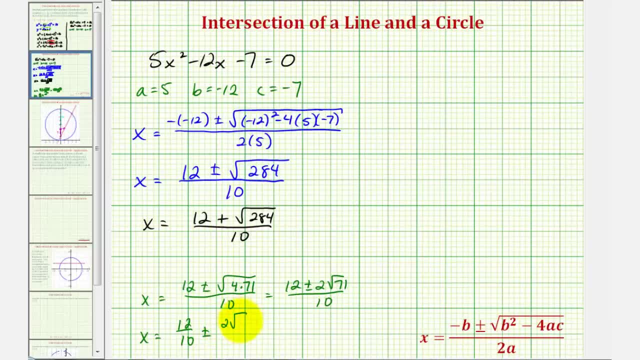 12 tenths plus or minus Two square root of 71 divided by 10, which would give us six-fifths plus or minus the square root of 71 divided by five, And of course we could write this as a single fraction if we wanted to. 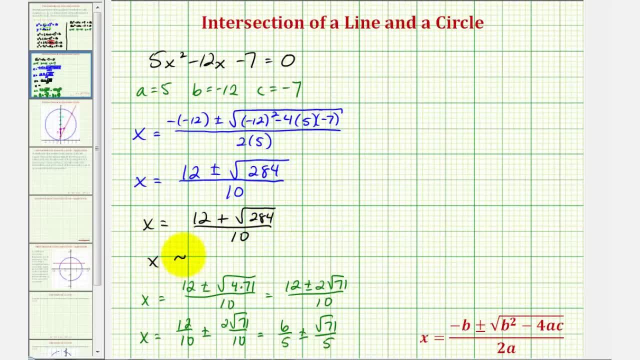 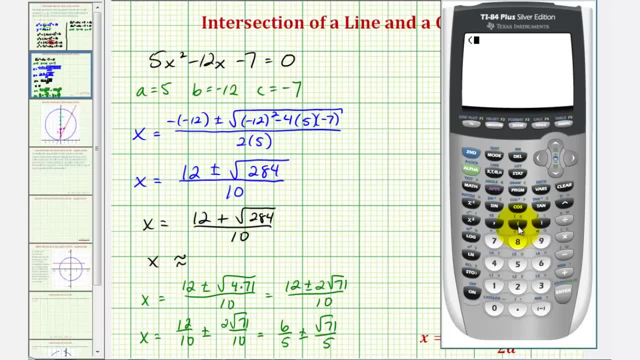 But again, for our purposes, we're only concerned about the decimal approximation of this to three decimal places. So using a calculator, so we'd have open parenthesis for the numerator 12 plus the square root 284.. Close parenthesis for the square root, another one for the numerator. 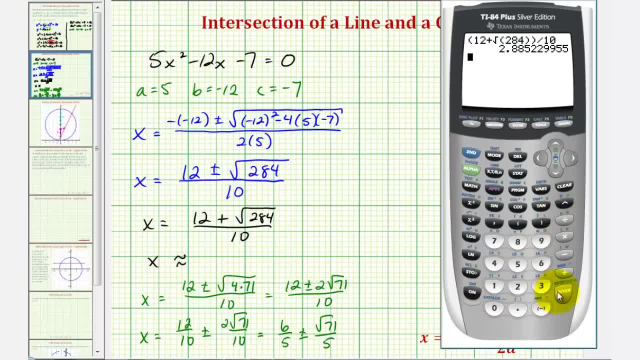 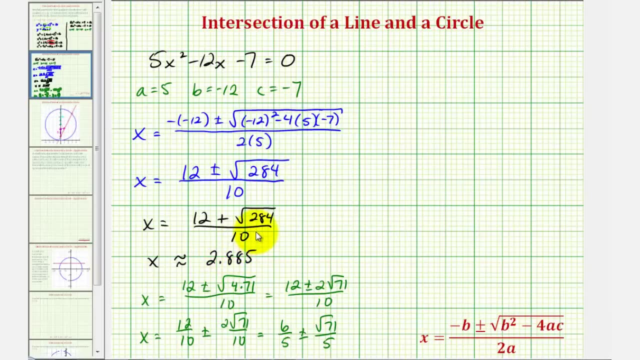 and then divide it by 10.. So x is going to be approximately 2.885.. Notice how the fourth decimal place is a two, indicating we round down, So x is approximately 2.885.. We still have to find the y coordinate though. 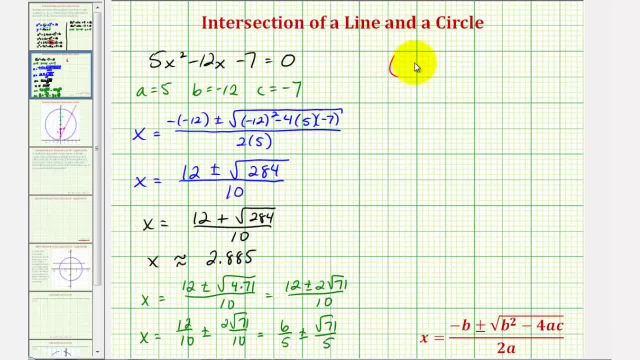 And we know that the point of intersection in the first quadrant has an x coordinate that's approximately 2.885.. And now to find the y coordinate, perform back substitution. Let's go ahead and use the linear equation, which was: y equals 2x plus 1,. 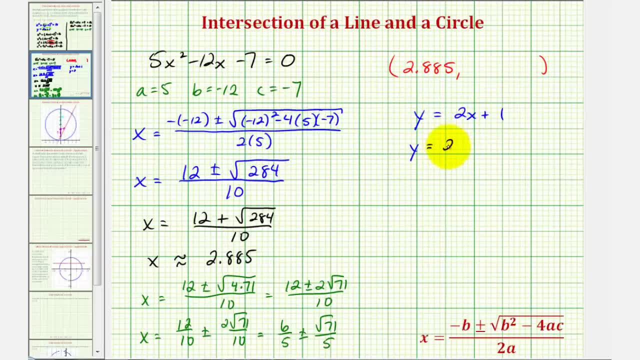 to find the y coordinate. So we'd have y equals 2 times 2.885 plus 1, which comes out to y equals 6.770.. So this would be the y coordinate of the point of intersection. And again, keep in mind these have been rounded to three decimal places.